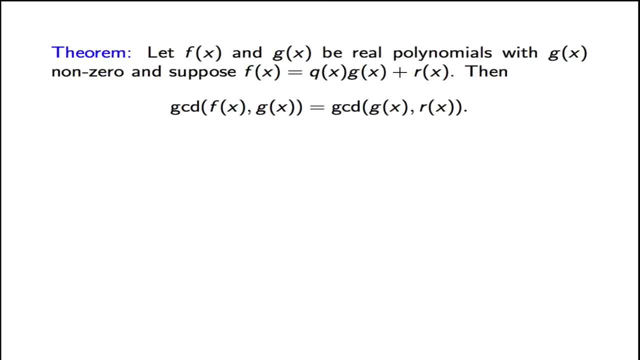 common divisor is completely analogous to the result we had for integers, Namely if f and g are two real polynomials with genome 0, and f is equal to q, g plus r, then the greatest common divisor of f and g is equal to the greatest common divisor of g and r. 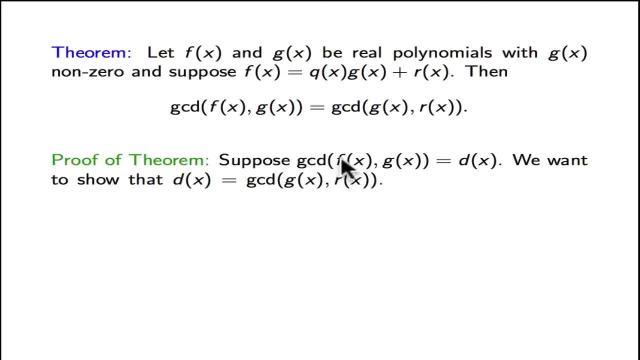 Let's proceed with the proof and let's suppose that the greatest common divisor of f and g is equal to d, and we want to show that d is also the greatest common divisor of g and r. So, indefinitely, d is monic. That's one of the conditions. 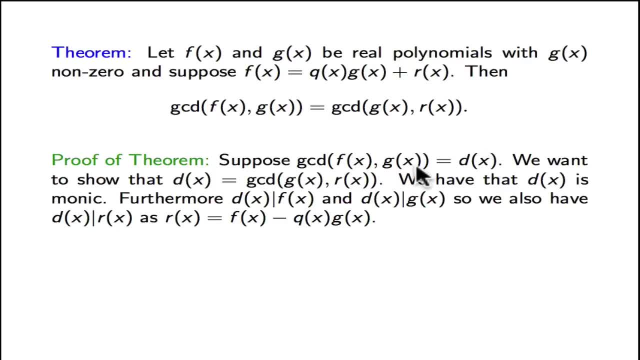 Secondly, since d is the greatest common divisor of f and g, it divides both f and g, And so it must divide r as well, because r is equal to f minus q, g. So d divides g and r, and the only thing that remains to show is that if some h 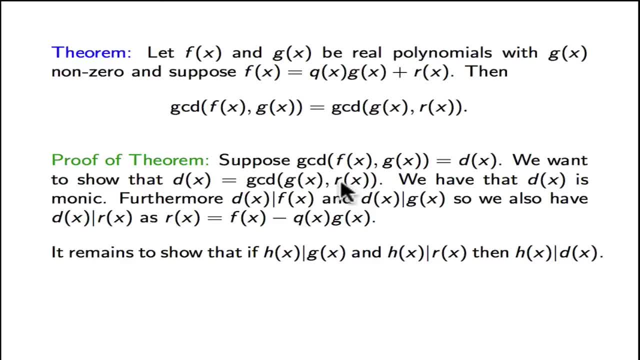 divides g and r, then it divides d. So it remains to show that if h divides g and r, then it divides d. But because f is equal to q, g plus r and h divides both g and r, then it must divide f. So we know that h divides both f and g. 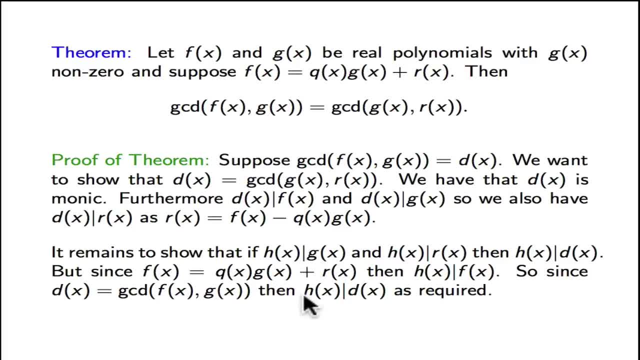 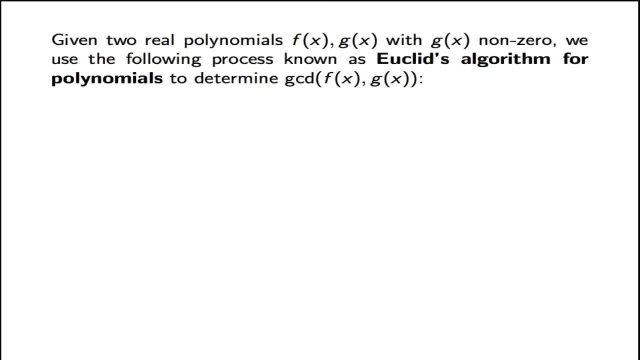 But d is the greatest common divisor of f and g, So h divides d, and this is what was required and the proof is complete. Okay, we are now ready to describe Euclid's algorithm to determine the greatest common divisor of two polynomials, f and g, and we suppose that g is non-zero. 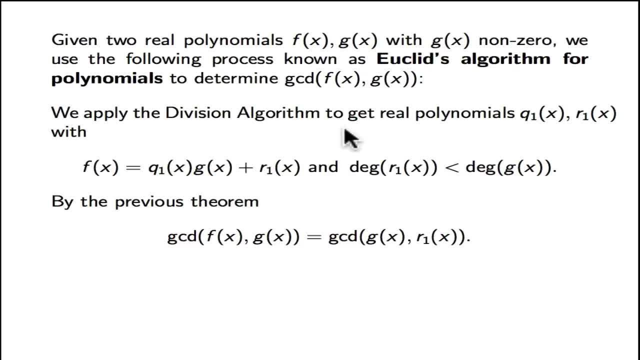 Okay, firstly, we apply the division algorithm, So we get real polynomials q1, r1, such that f is equal to q1, g plus r1, and the degree of r1 is less than the degree of g And the previous theorem. 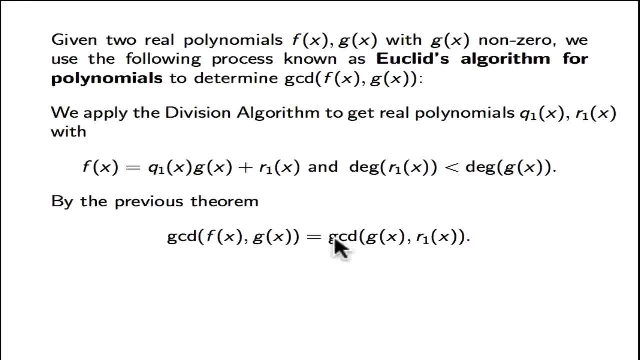 says that the greatest common divisor of f and g is equal to the greatest common divisor of g and r1. So it's enough to determine the greatest common divisor of g and r1.. If r1 is zero, then we stop, Otherwise we'll continue. 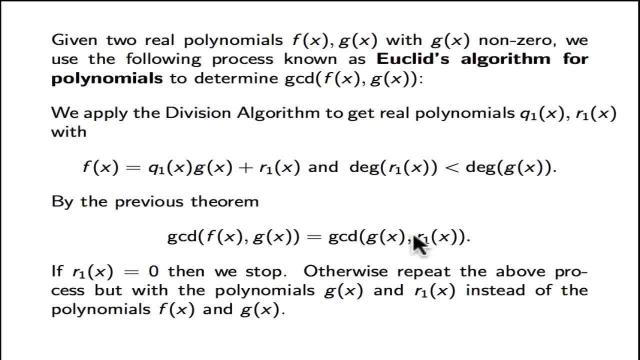 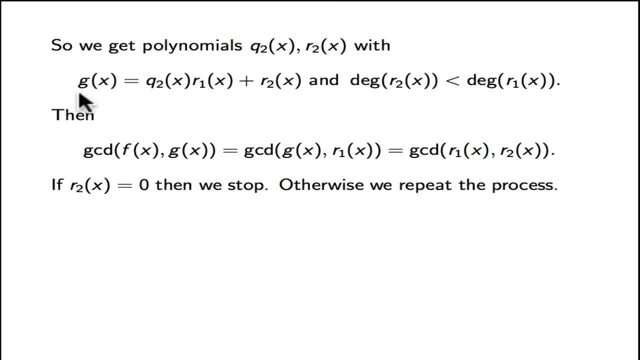 But we again repeat the process, but with the polynomials g and r1 instead in place of the polynomials f and g. So we get polynomials q2 and r2, with g equals to q2 by r1 plus r2, and the degree of r2 being less than the degree of r1. 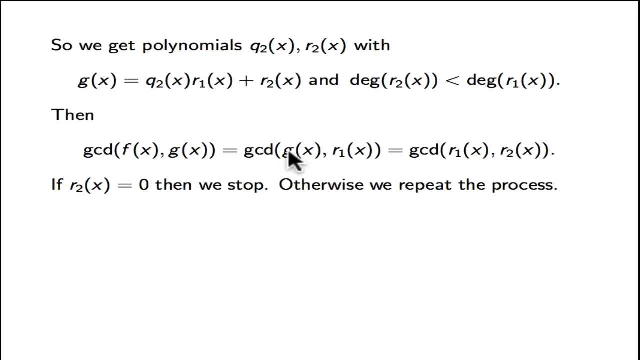 And then the greatest common divisor of f and g, which we have already shown. that is equal to the greatest common divisor of g and r1, of R1 and R2.. So it's enough to find the greatest common divisor of R1 and R2.. 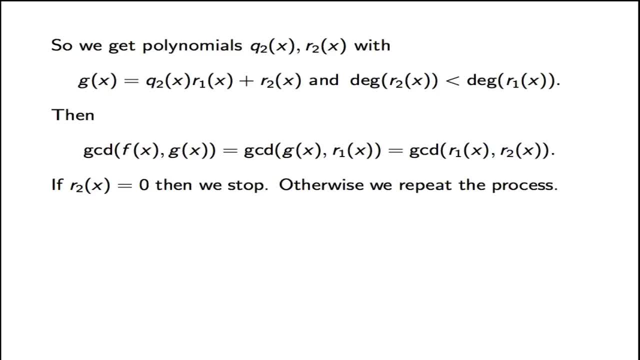 If R2 is equal to zero, then we stop. otherwise we repeat the process And at the kth step we will have non-zero polynomials- R1 of x, R2 of x, R2, Rk of x- with their degrees strictly decreasing and the greatest common divisor of f and g being equal. 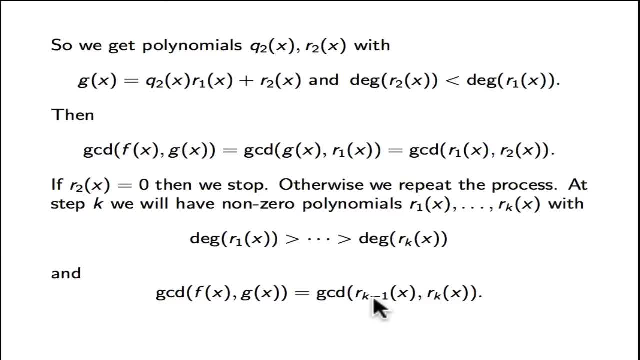 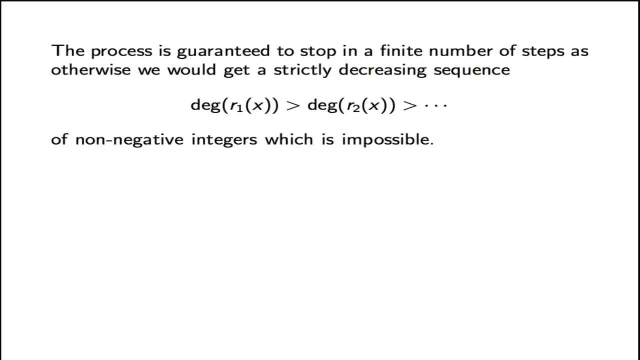 to the greatest common divisor of the last two R's, Rk-1 and Rk, And this process is guaranteed to stop in a finite number of steps, as otherwise we will have an infinite, strictly decreasing sequence of non-negative integers, which is impossible. But then, if it stops at the nth step, 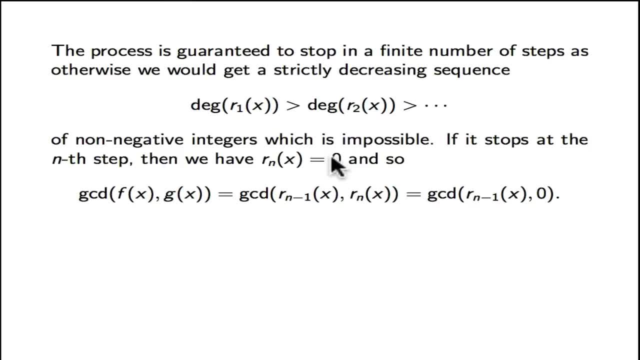 ie if Rn of x is equal to zero, then we know that the greatest common divisor of f and g, which is equal to the greatest common divisor of Rn minus Rm, is equal to the greatest common divisor of Rn-1 and zero. 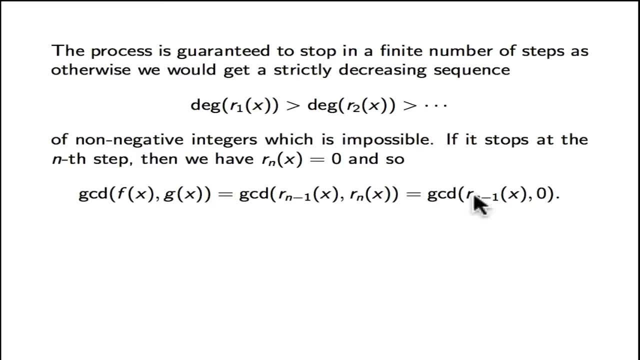 Now we need to take some care. It's not the case that the greatest common divisor of Rn-1 of x and zero is equal to Rn-1 of x, as it was the case when we were dealing with integers, And the reason is that Rn-1 of x may not be 몽, But if Rn-1 of x has leading coefficient, a, 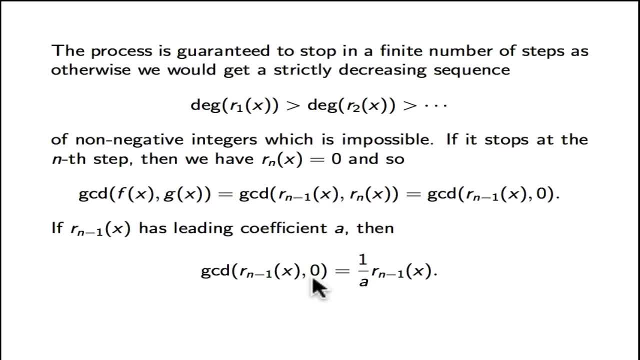 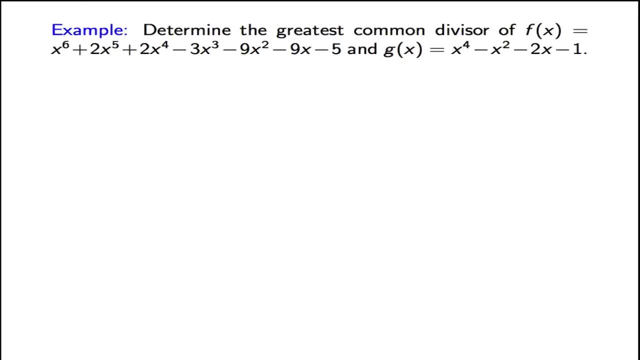 then the greatest common divisor of Rn-1, one of x and zero, is actually equal to one over a times r n minus one of x. So let's see this in practice and suppose we have these two polynomials, f and g, where 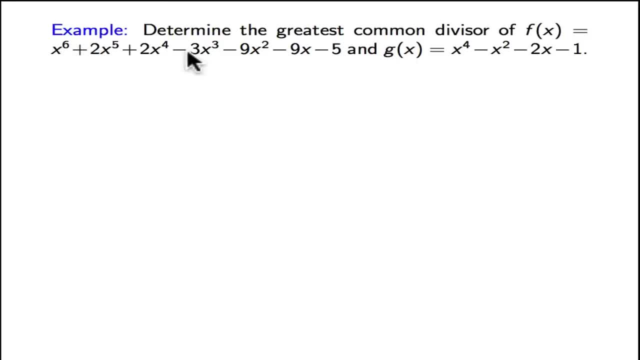 f is equal to x to the six plus two, x to the five, and so on. and g is equal to x to the four minus x square, and so on. So first step is to apply the division algorithm to f and g. Now I won't do the division algorithm, so I'll just write down the answer and we can. 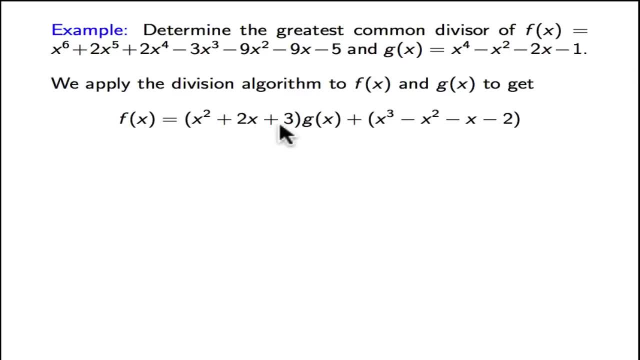 find that f of x is equal to x square plus two x plus three times g of x, and the remainder is x cube minus x square minus x minus two. Now, because this is non-zero, then we are going to apply the division algorithm to g. 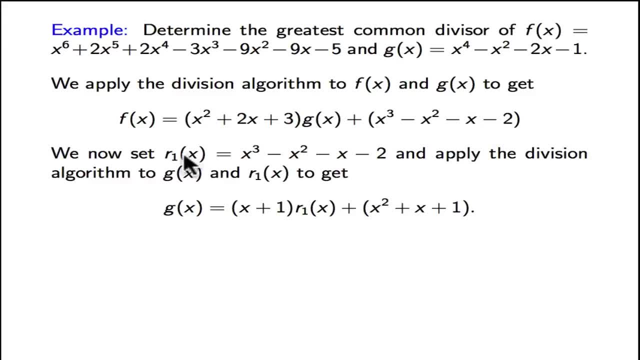 of x and this one. So let's first give it a name, let's call it r, one of x and let's apply the division algorithm to g and r one. And again, I'm not doing the division algorithm, I'm just writing down the answer and we'll. 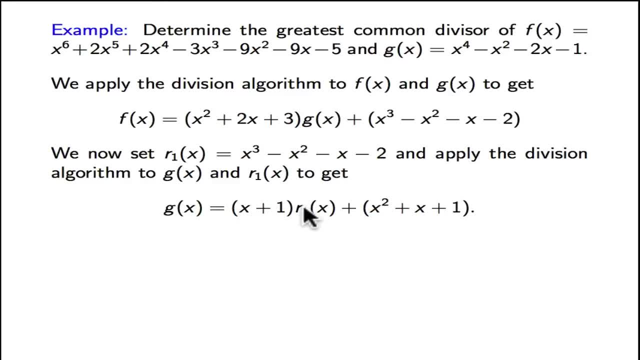 get that g of x is equal to one over a times x to the five, and so on. So g of x is equal to x plus one times r, one of x plus a remainder of x, square plus x plus one. So this is non-zero. let's call it r two of x and let's apply the division algorithm. 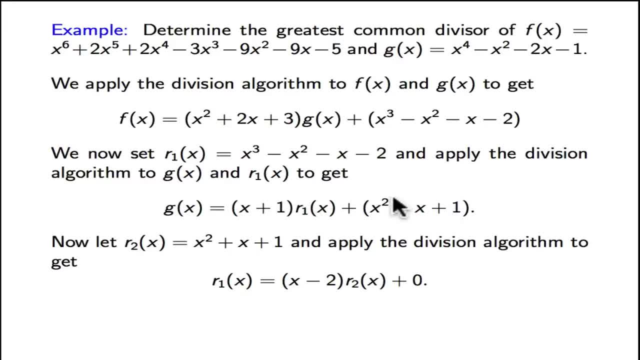 now to r one of x and r two of x, and what we get now is that r one of x is equal to x minus two times r two of x plus zero. So now we stop, And the greatest common divisor is a suitable multiple of r two of x, so that it will be: 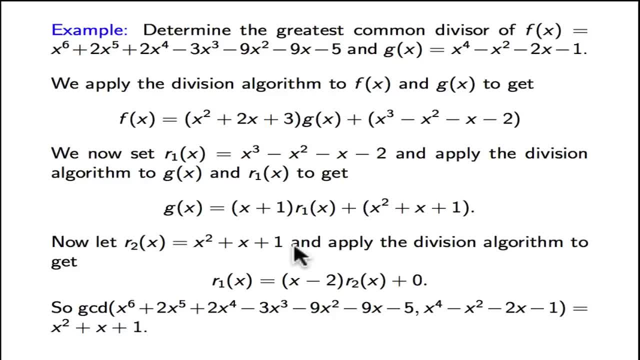 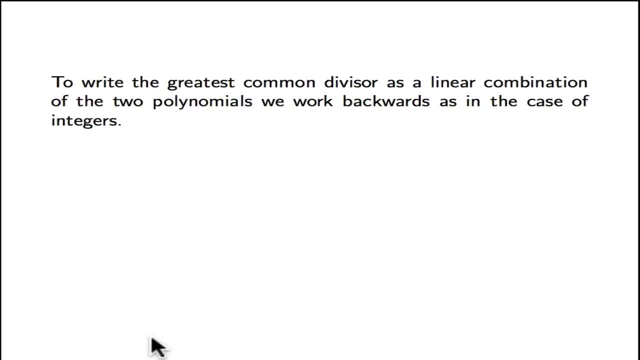 monic, but r two of x is itself monic. so the greatest common divisor of the two polynomials is x square plus x plus one. And, as in the case of integers, if we want to write the greatest common divisor as a linear combination of the two polynomials, we walk backwards. 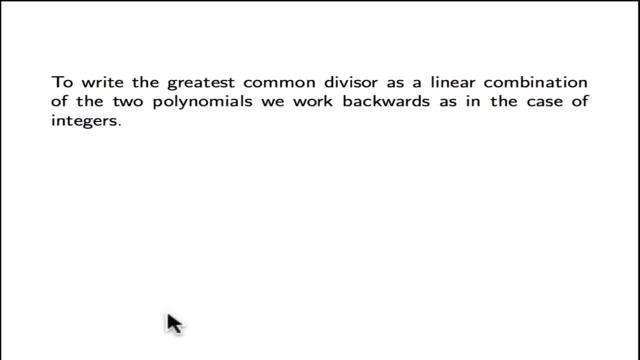 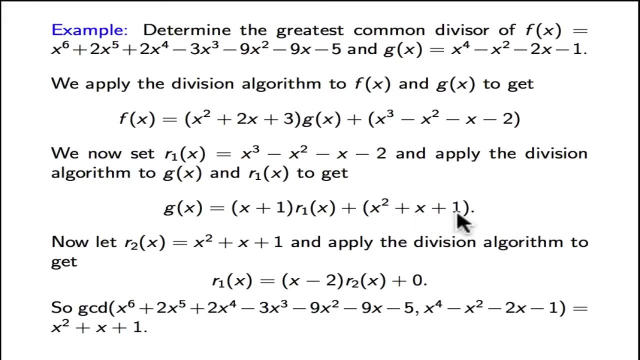 So in the previous example we have the following: So we start with this last equation. We know that x square plus x plus one is the greatest common divisor. We want to write it as a linear combination of f and g. So the first thing we do is to write it as a linear combination of g and r one. 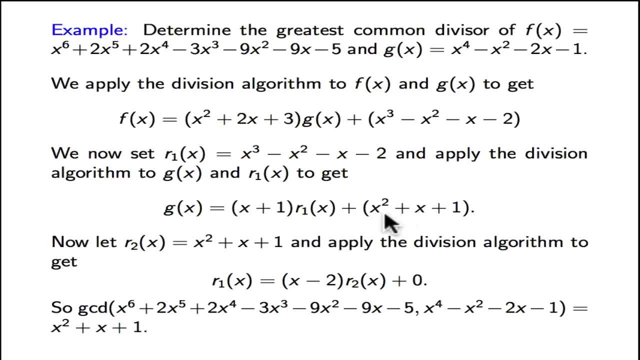 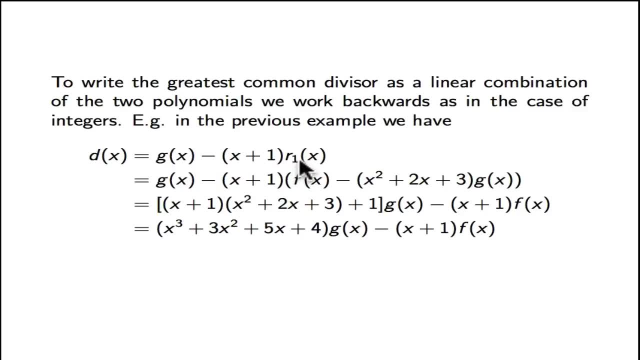 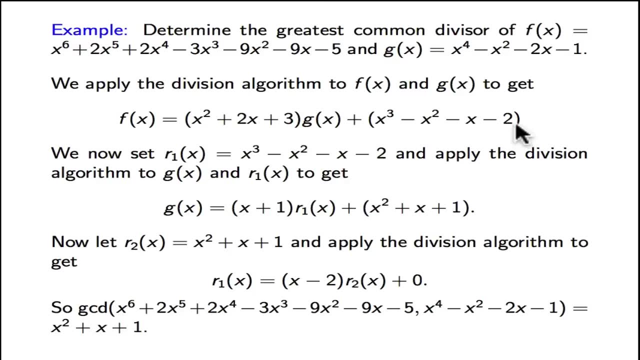 So the first step is to write d of x being equal to g of x minus x, plus one r one of x. This is what we did here. Now we take r one of x, which is this one, this polynomial here, This polynomial r one of x. we can write it as a linear combination of f of x and g.